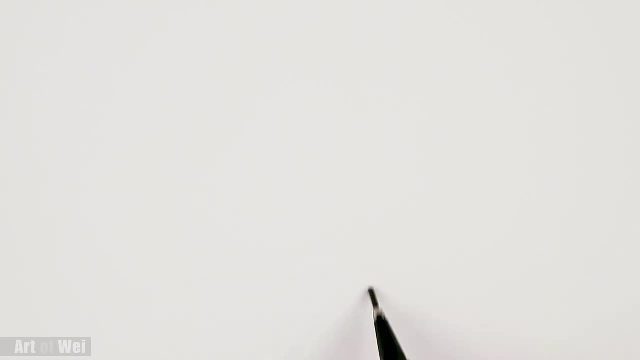 All right. so to draw any kind of cone, an easier way to draw it is to just draw in a little bit of elliptical first- Okay, so this would be the base, And then from this elliptical you just draw in a line all the way across the widest part. 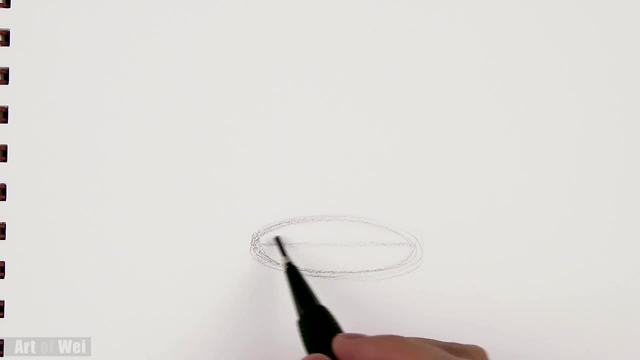 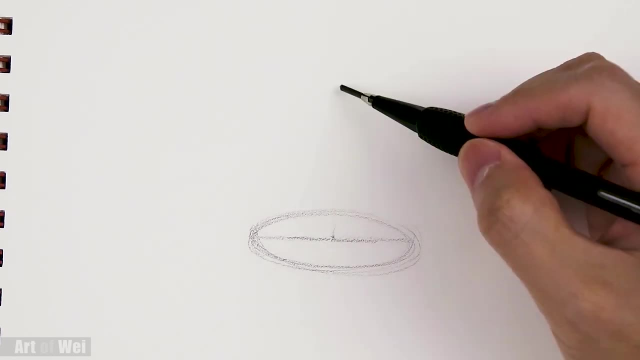 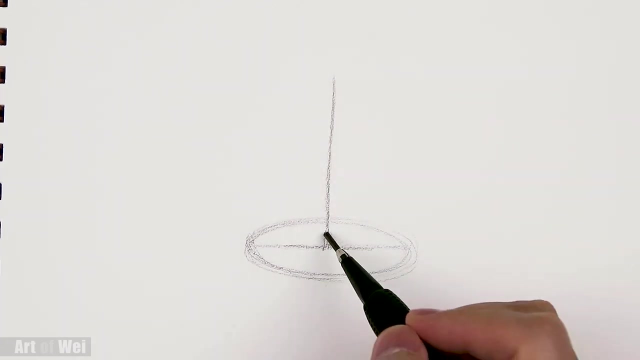 That's going to give us kind of like you're cutting it in half And then come to the center of this And then whatever line you have here, just draw a little right angle. We'll go straight up. Mine is a little bit wobbly, so this would be a right angle. 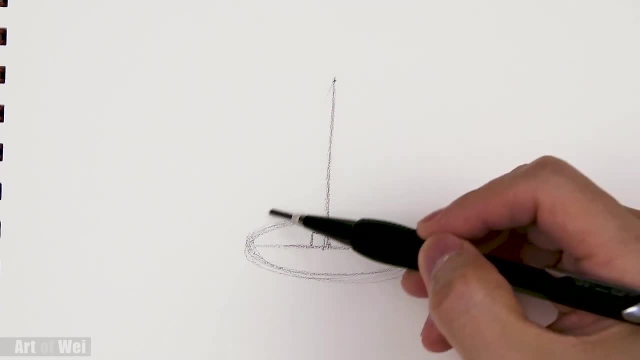 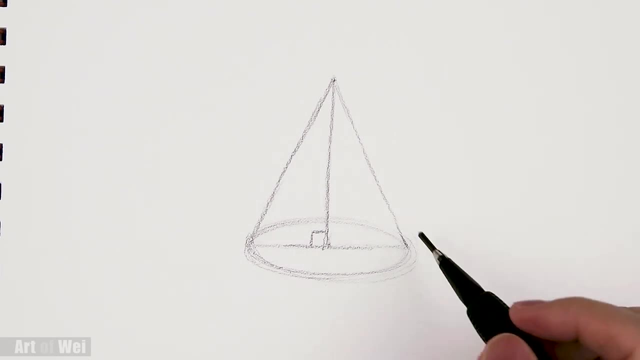 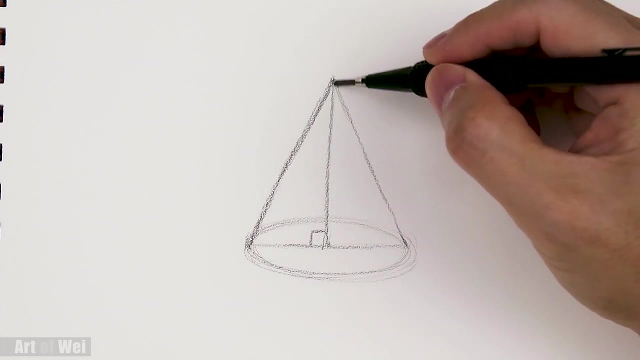 And then, once you have that from the tip here, just draw a line all the way to the edge, Okay, so yeah, it actually looks kind of like a boat, right? Okay, so I didn't see that coming, All right, and then let's see. So that would be the edge. Now I'm just going to round it out. 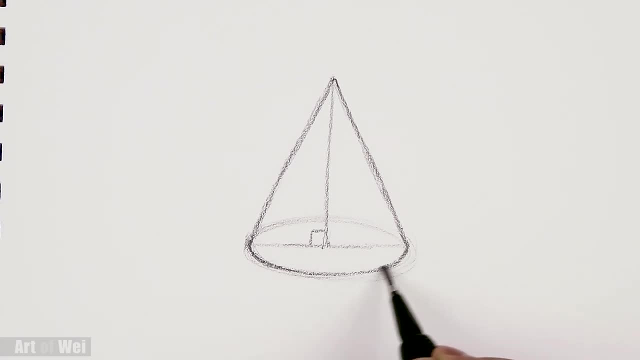 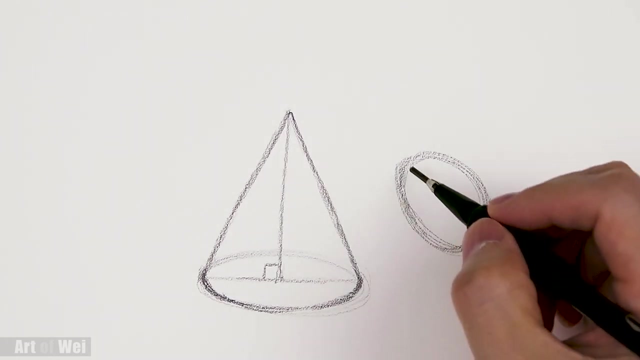 Just clean this up a little bit And that's going to give us a cone, Or so you can draw it in any kind of direction. Let's say you have maybe a little bit wider. Okay, let's try to freehand an ellipse, which is always kind of difficult. 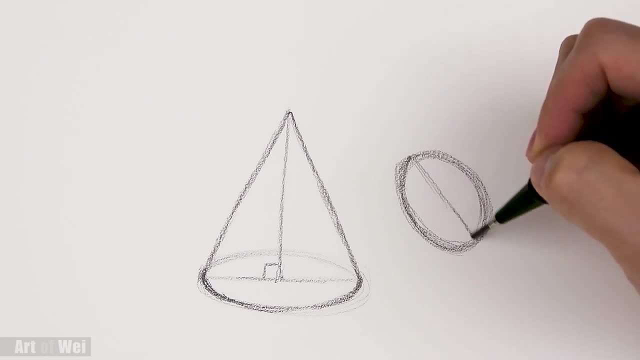 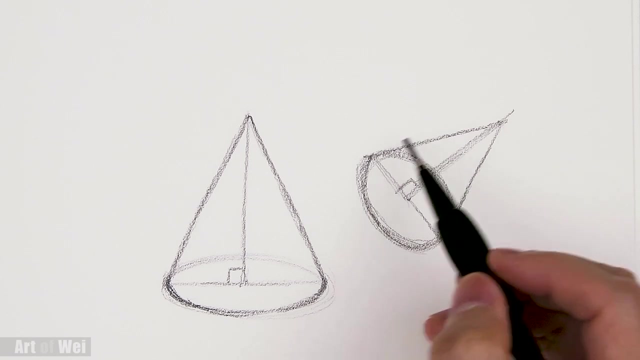 All right, and then from here just the widest point, One line across, And then from the middle, Again 90 degrees right here From the tip, however high you wanted to make it, So that would be your cone again. So here's the edge. 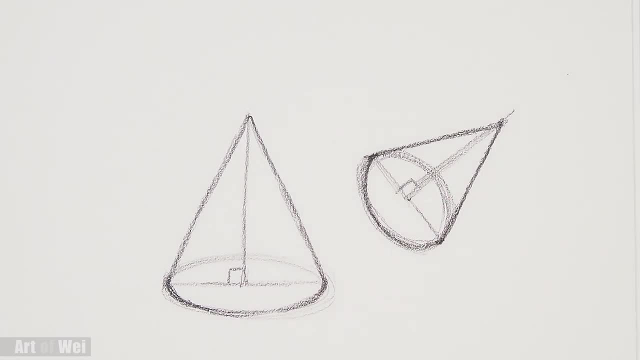 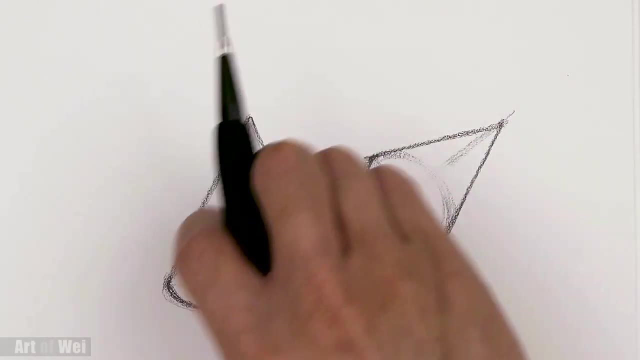 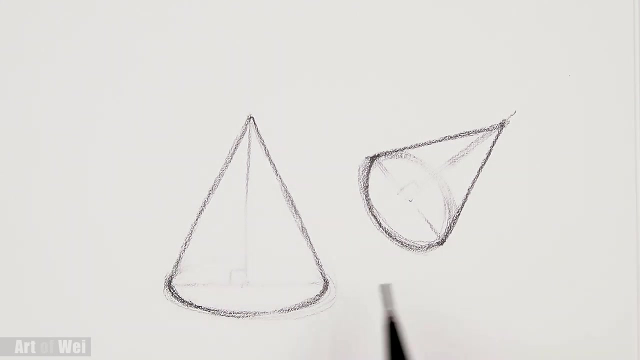 Just going to round this out. Okay, so then you can just kind of erase out the lines on the inside here, Then we can see it clearly. All right, so whenever you draw this kind of shape, always just go ahead and draw in the back too. 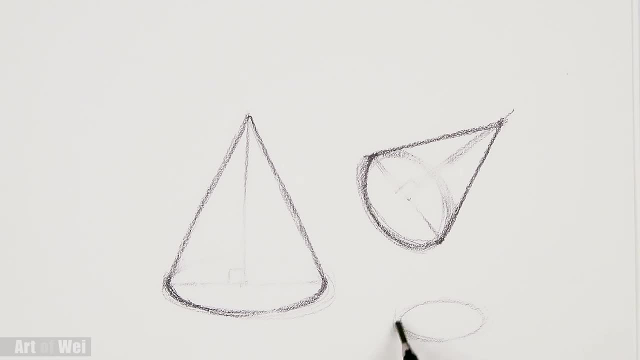 You know, we always want to envision the full shape, even behind it, And that's going to give you- you know just a little, I guess- better representation of you know what you're trying to draw And you're going to feel the shape a little bit more. 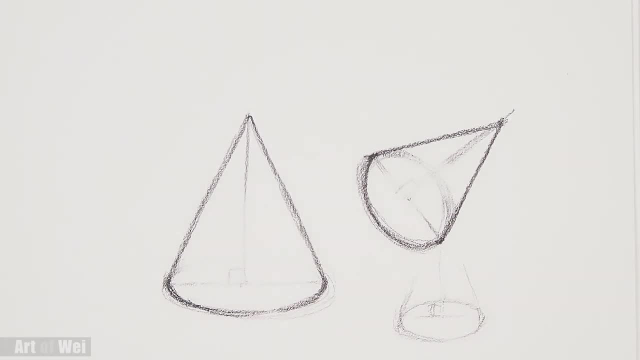 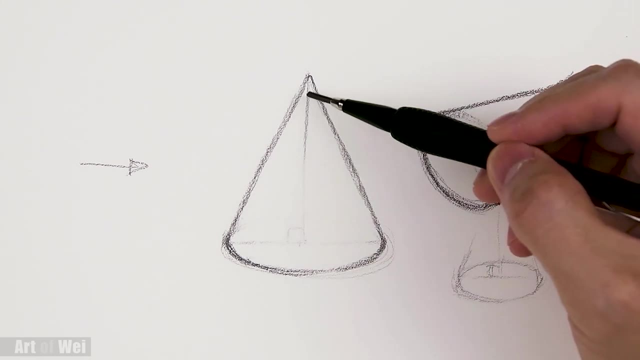 Okay, so for shading, let's come back to this shape so that we don't have to draw it again. Okay, So let's just say that there's a light coming through this side. Okay, so, here, from the center, right here, I'm just going to go straight down. 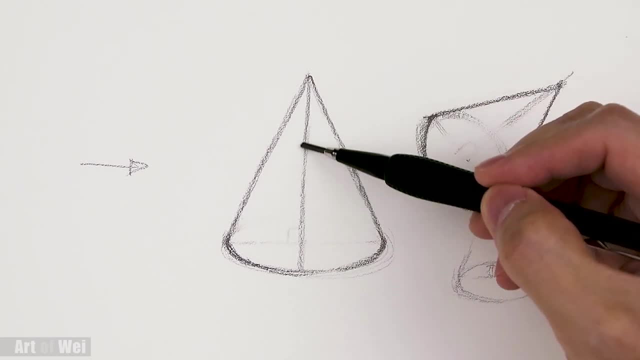 And this can be anywhere. I'm just trying to make it easy. So it's just right in the center, right here. So that means the light's coming here. This will be the terminator right here, So the light's going to fall off. 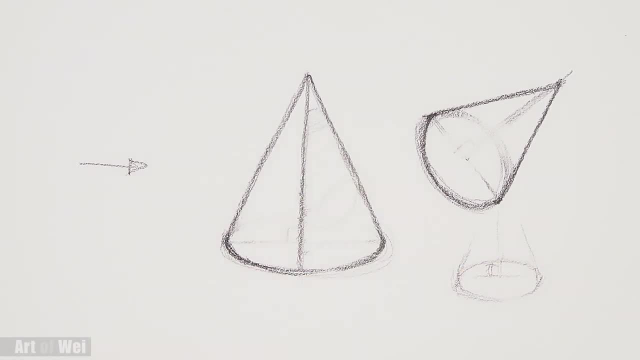 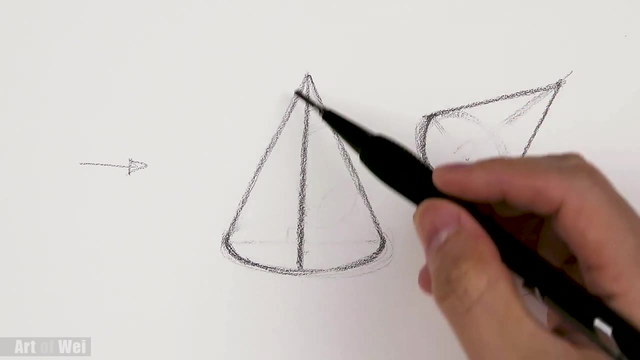 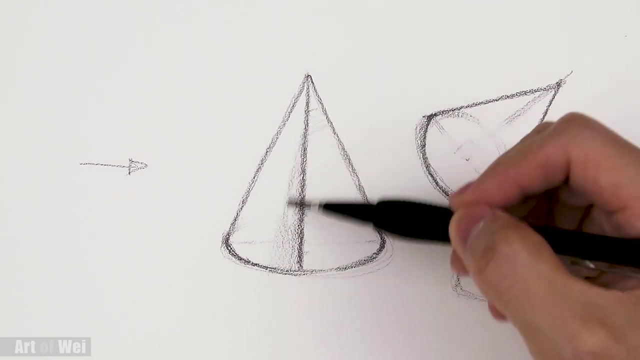 And on the back right here. this light's not going to reach any of this area. All right, so we can make this kind of dark. Now I'm going to shade this side first, So from this part I'm just going to go this way. 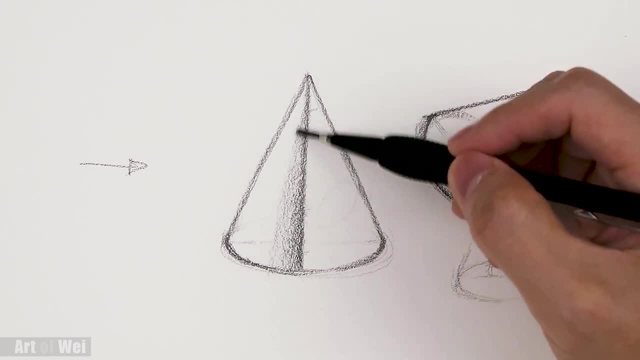 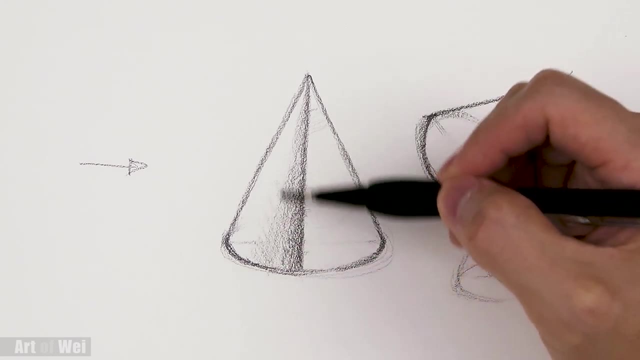 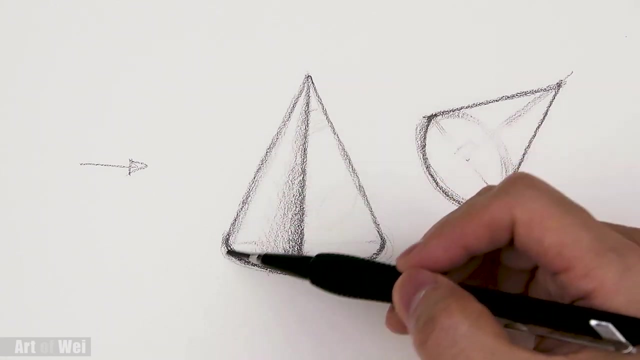 Make this a little bit darker here, Okay, and then from here let's just even it out just a little bit more, Let's say the highlight's right around here, And then on this edge, I'll shade in a little bit, because this, you know, we want to show this being round. 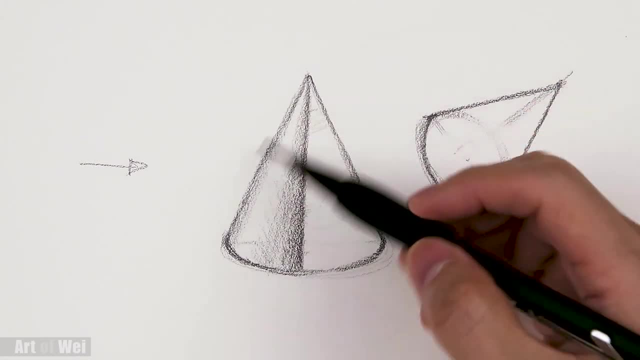 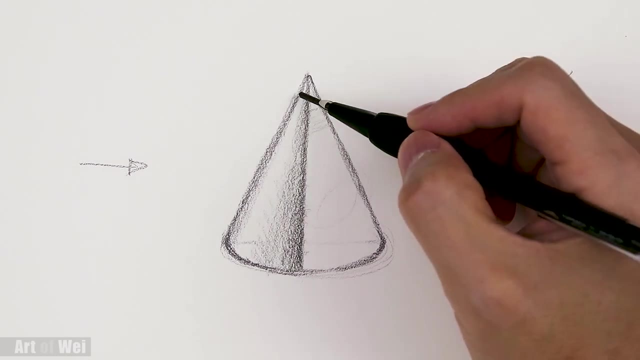 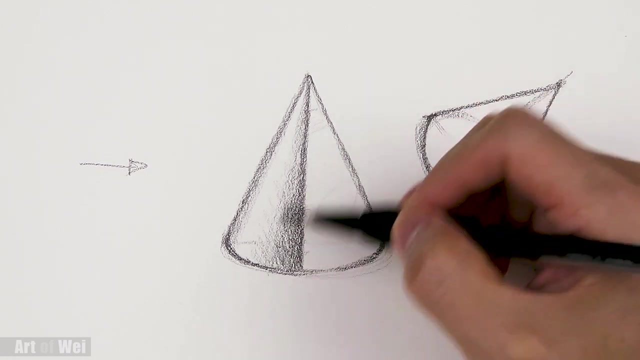 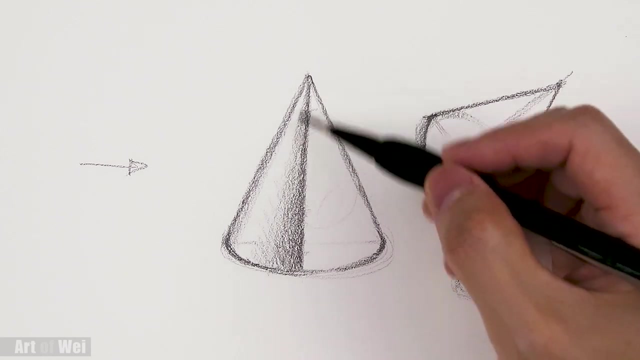 And it would be a little bit darker right here, And I'll talk about some of the more important things about shading this a little bit later. Let me finish shading this first, Because there's a lot of a common error on shading. the cone is actually drawing shading on the top right here. 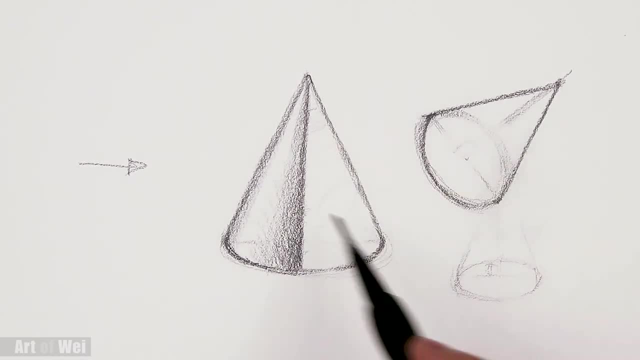 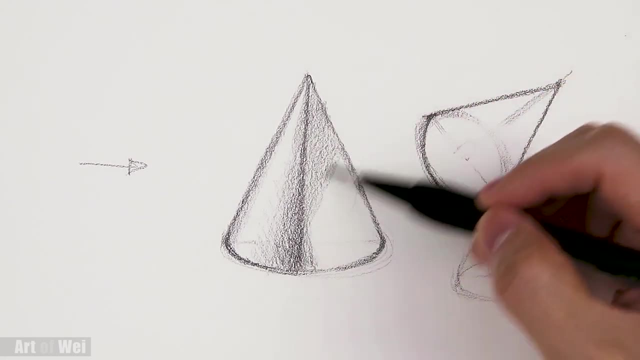 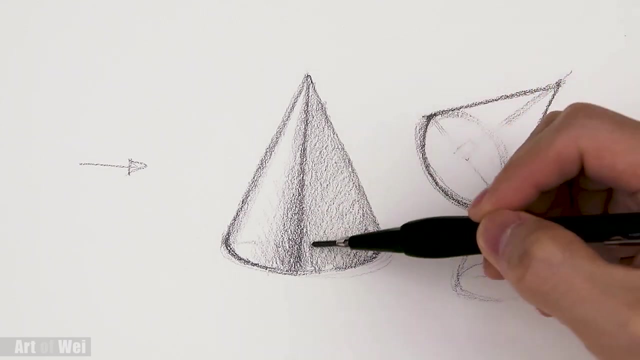 Okay, so that's going to be the front, And then now for the back. So whatever light you have here, So let's just continue this. I'm just going to give this an overall darker shade first. So the thing to remember: whatever happens back here has nothing to do with this light coming this way. 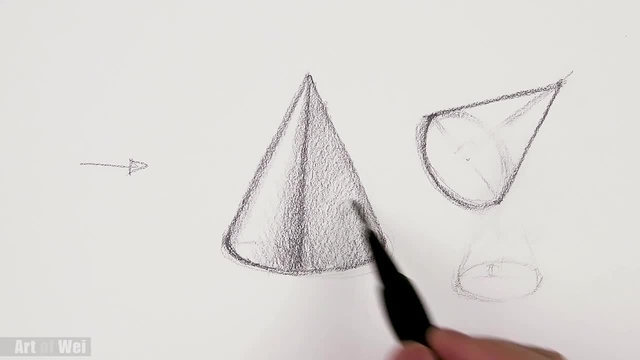 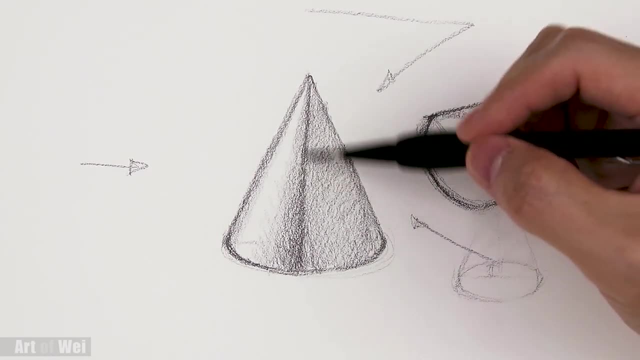 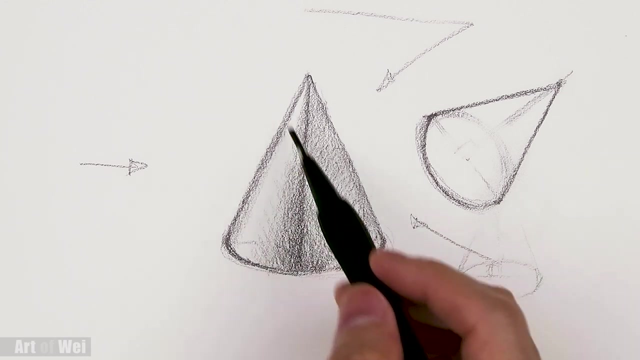 It has everything to do with the light going past and hitting the environment and bouncing back into this. So this is going to be all based on bounce lighting, All right. So in general, we want to make this a little bit darker And then this we got. actually, it's going to be the same kind of shading as this, but just on this side. 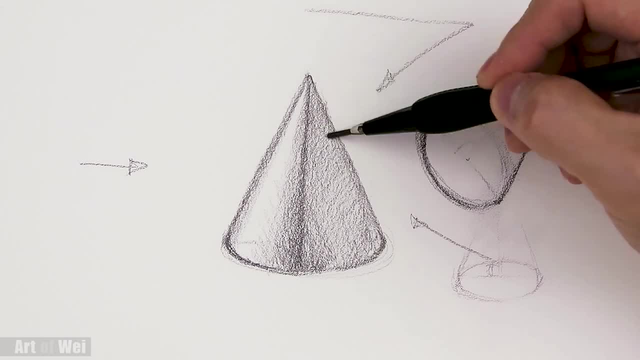 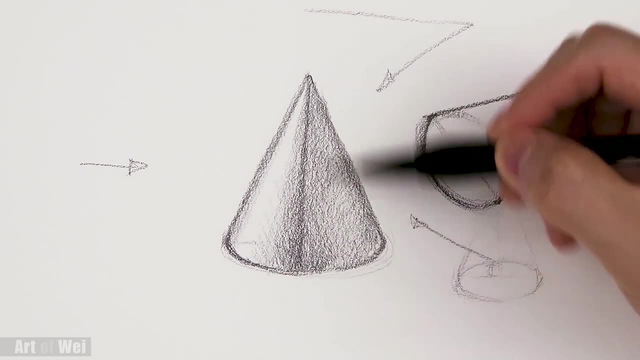 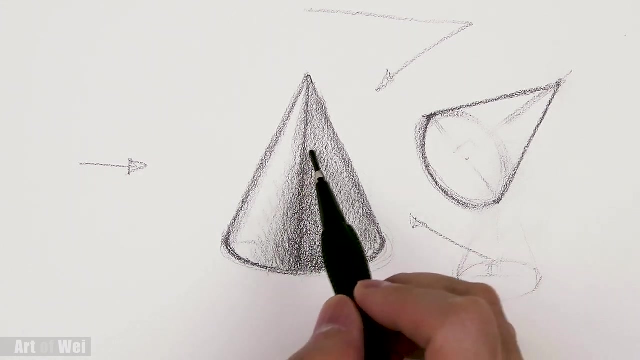 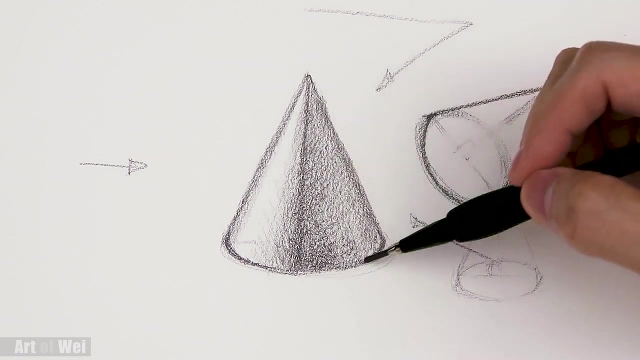 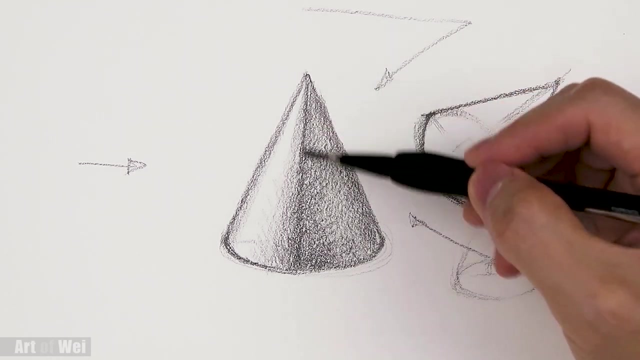 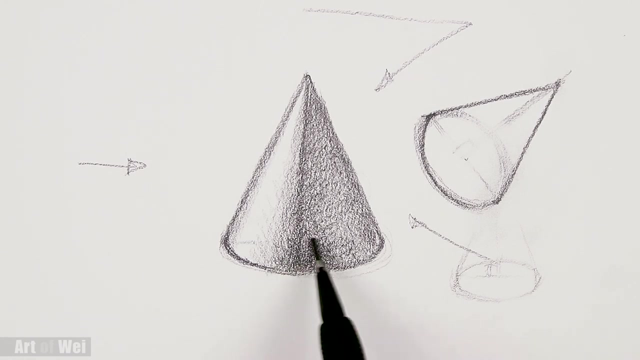 But everything's going to be darker. So I'm going to shade this way: Just a little bit of cross hatching, A little bit darker here, Maybe even darker. It just depends on you know how much bounce light you want to make it or simulate it. 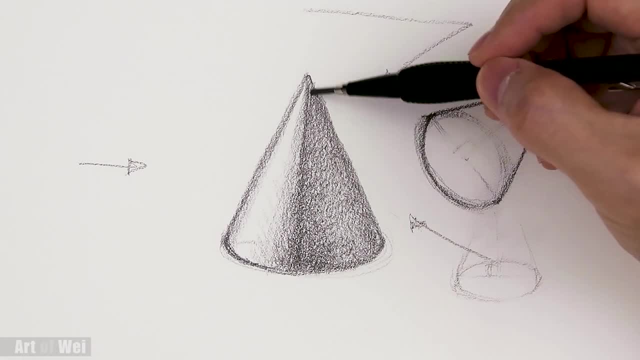 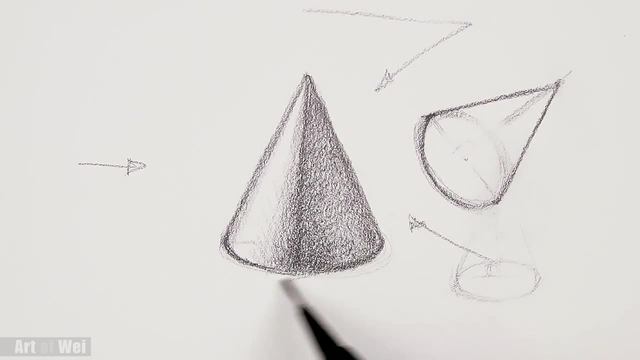 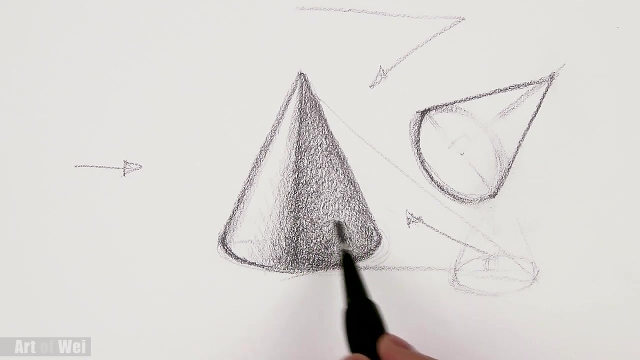 So if there's a lot of bounce light, obviously this will be a little bit lighter, Everything will be a little bit lighter, All right, And then let's see. if you want to draw the shadow, I'll just draw a real quick shadow right here. 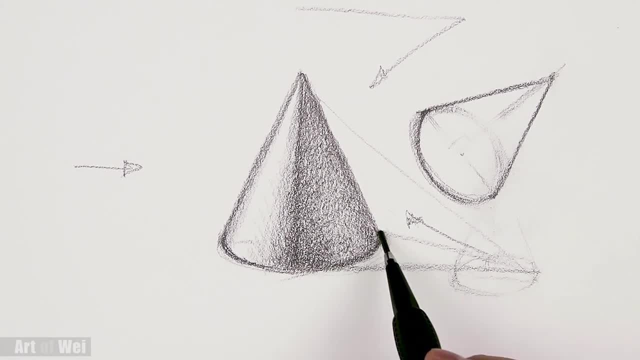 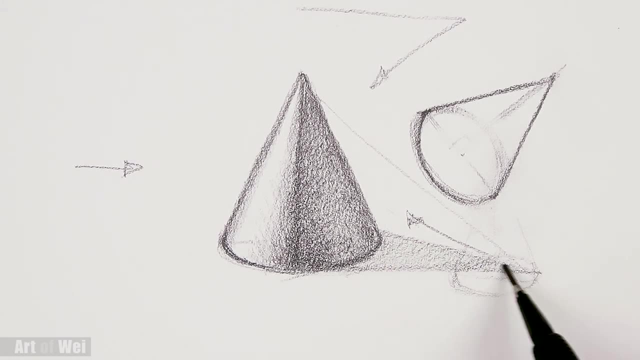 I'm not going to go into that much, because if you take any kind of perspective drawing classes, they'll show you how you can measure and draw these lines with shadows and stuff, All right, Just roughly, just something like that. Okay, So here's the important part about shading a cone. 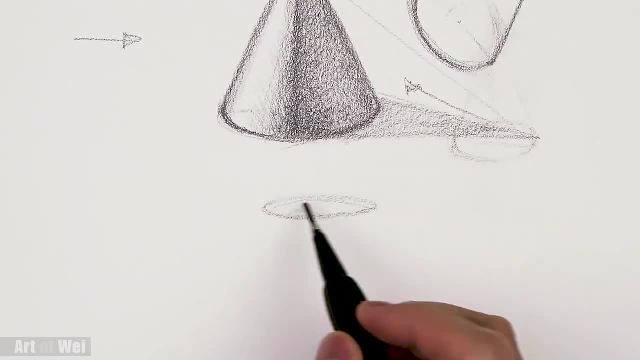 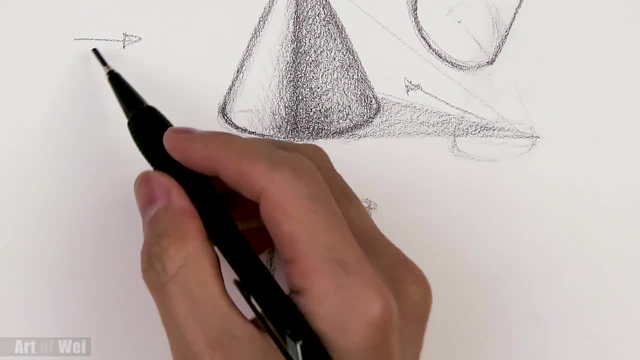 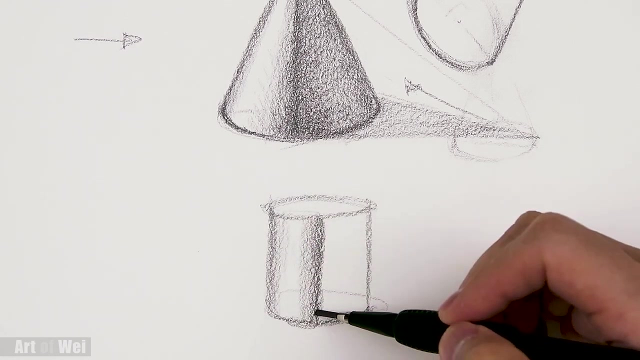 It's pretty much like shading a cylinder. All right, You have a cylinder, All right. So here's the middle. again, Again, same lighting, And this would be, you know, going to this, Here's the highlight. This will be the darkest part. 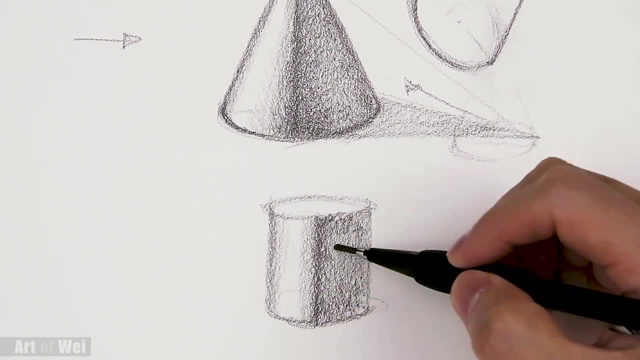 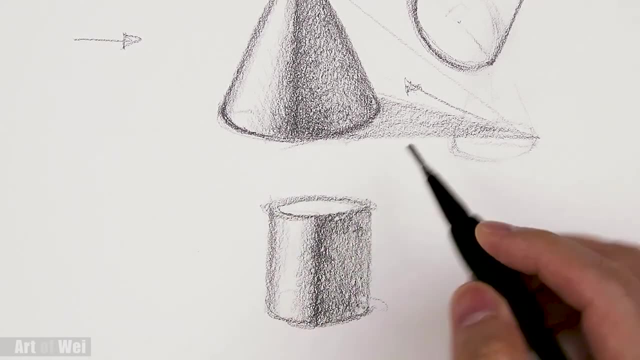 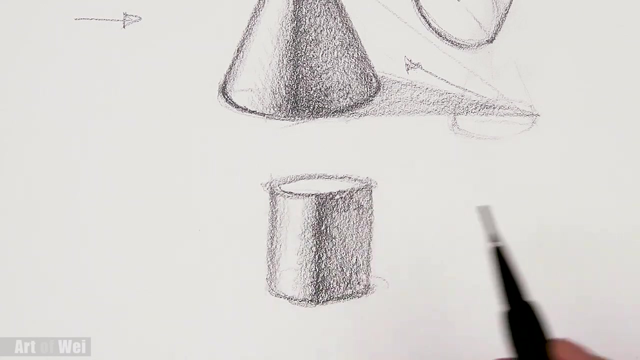 Give this one shade on the back first, And then again the bounce lighting. whatever you want to do, Smooth this out a little bit. Okay, So that's a cylinder, And the thing to remember is just that the cone is the same thing. 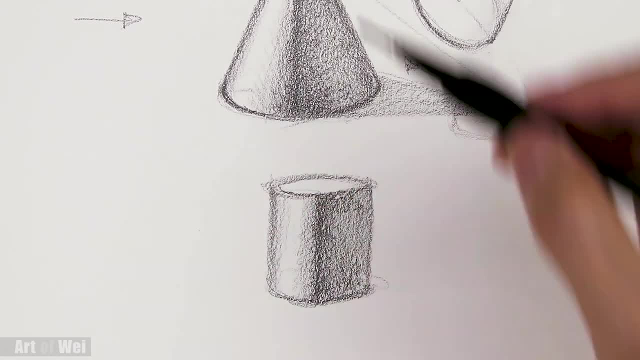 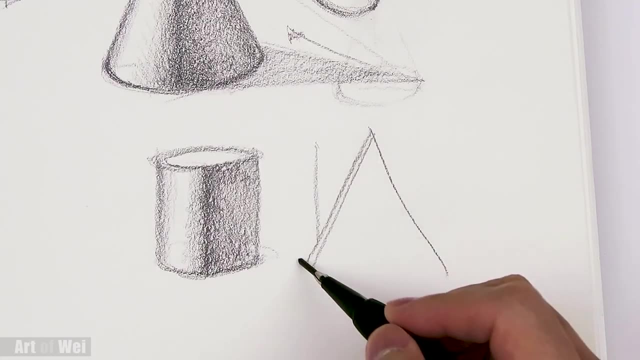 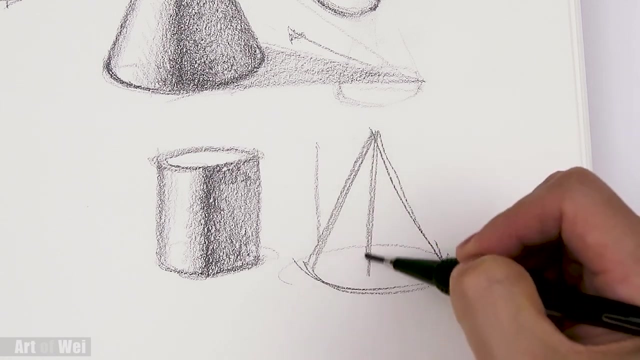 It's just that we're taking the upper part and we're squeezing it really, really small. So that's why, when you're shading this, say, let's see, let's move to here, Let's have this When you shave. so when you shade any section here, just remember, whatever you do down here has to be the same up here. 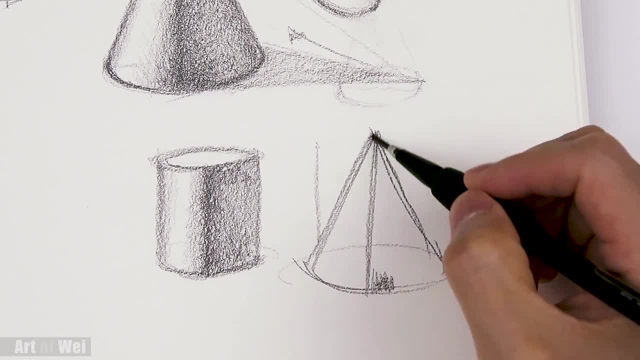 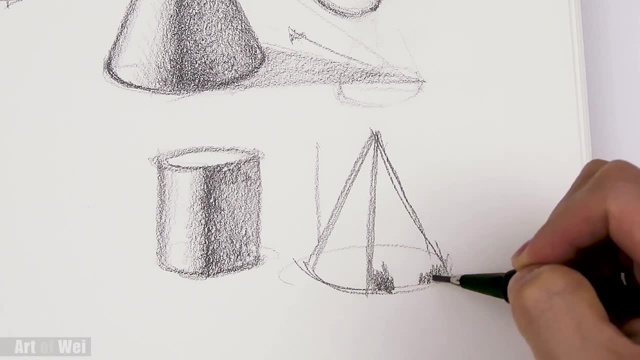 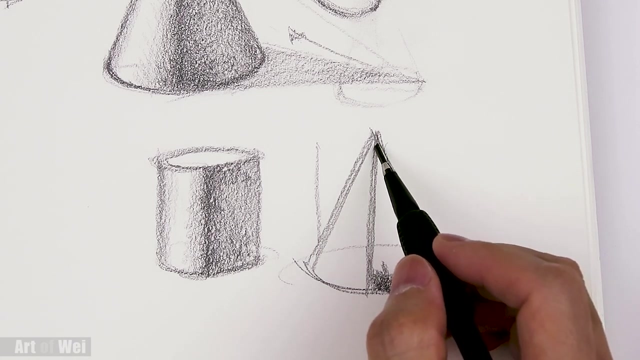 And it's going to be a lot smaller. Okay, So let's say, if you're drawing this really dark right here, Whatever You know shading you have up down here, you're going to have to replicate it up here, But it's going to be really, really tight. 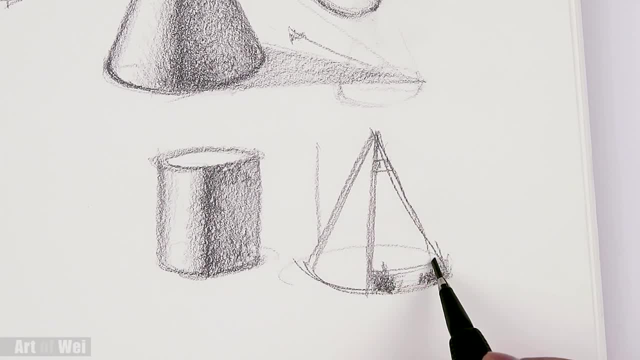 So you've got to take any kind of section here. If I take this section and I put it up here, it's going to be like that, right, It's going to be here, It's going to be right around here. Do this? 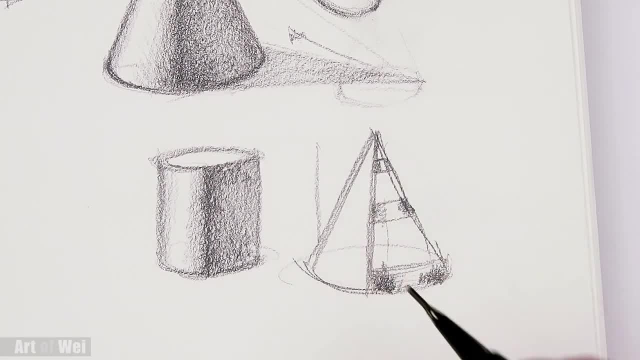 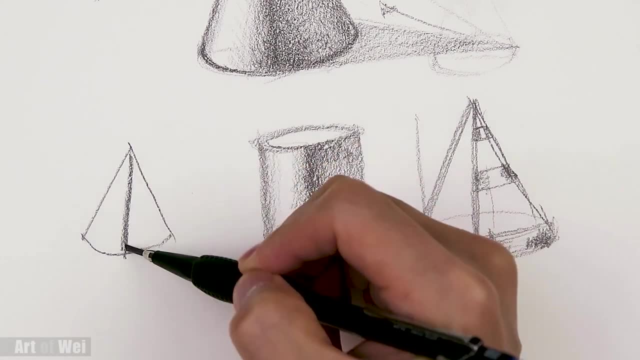 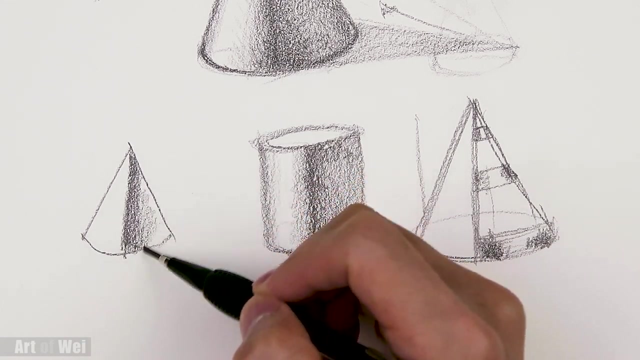 So that's the key part about shading. a cone is up here, Because a lot of time what happens is that you know when you're going to shade the top. you'll shade like this And then you're going to end up getting the top right here really dark compared to the bottom. 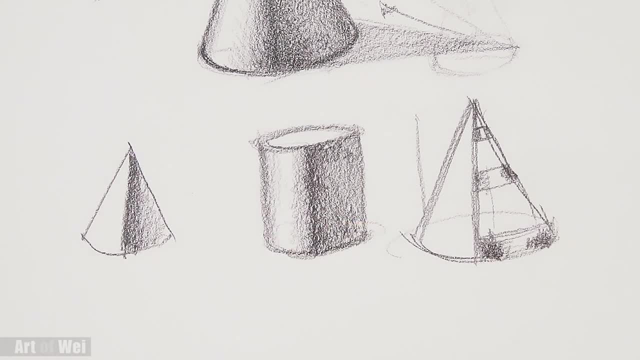 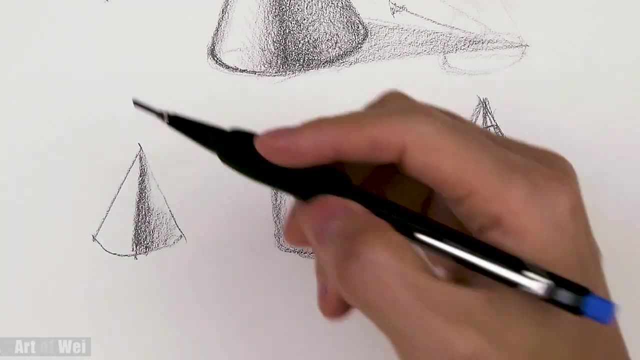 All right. So this looks a little bit weird, right? because it's a little bit too dark up here. So, right on the top, this is not correct. So this part right here needs to be a lot lighter Or the same kind of gradation. 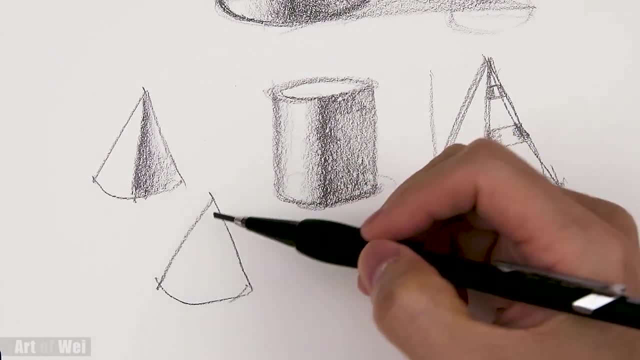 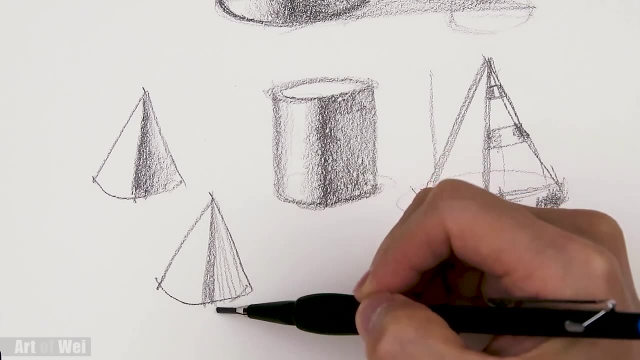 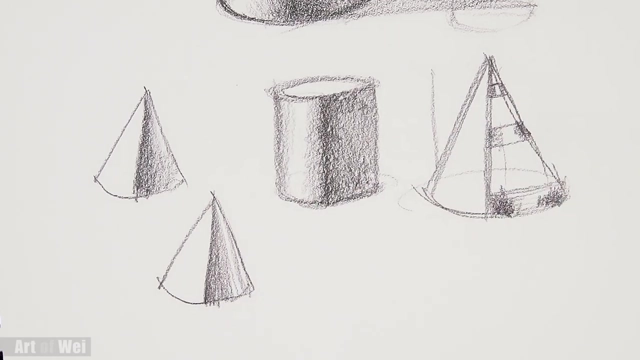 So I guess the easy way of shading a cone is to draw these kind of lines like this. It's almost a little fan, Okay. So it's more like this. Okay, So that the tip here don't get all you know, a little bit too dark. 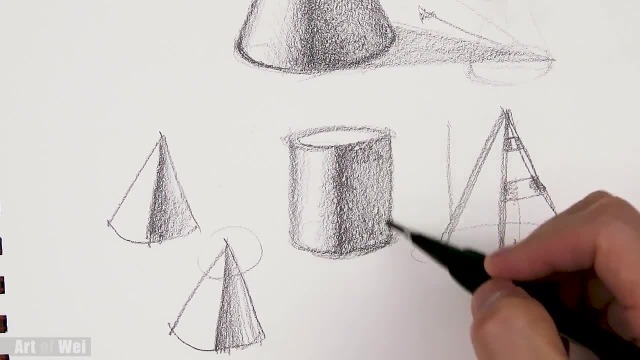 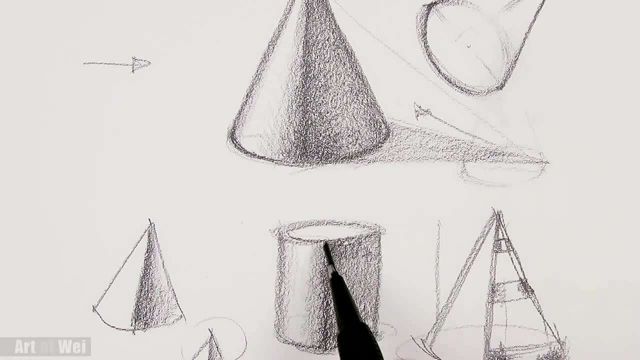 But that's the only thing I mean. everything else is pretty basic. So just kind of remember, It's the same thing as the cylinder: All we're doing is just squeezing the top. So all this space right here gets squeezed to a really small area right there. 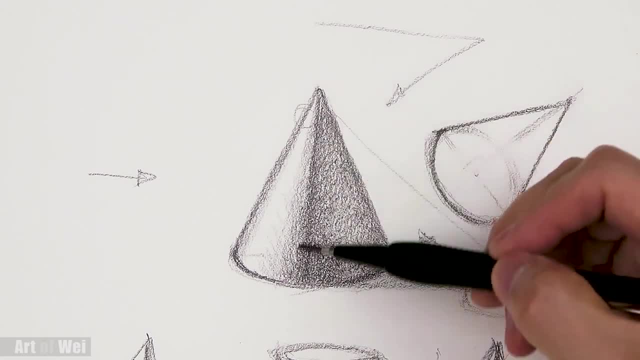 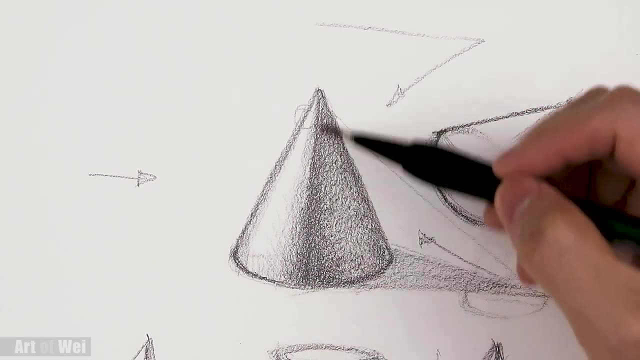 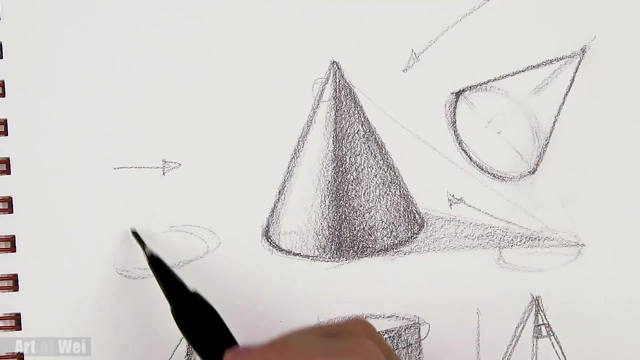 And that's the same. You know it goes the same thing on both sides. Okay, So I think that is pretty much it. You know, these are very basic shapes And again they're very important to kind of understand and just kind of be able to freehand it.